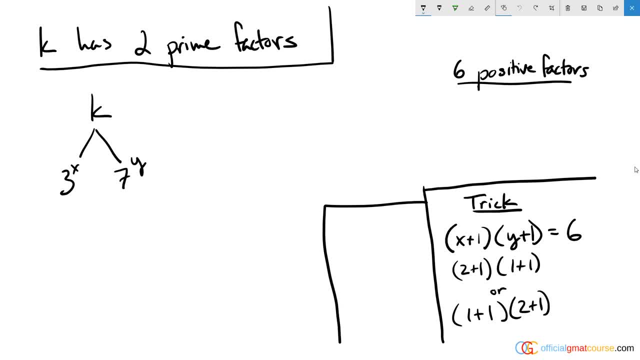 example which doesn't follow the exact rule that we've been given in this question, but has a similar principle behind it. So the example is going to be the number 12.. And if we factor the number 12, we see it has factors of one and 12, two and six, and three and four, So it has a total. 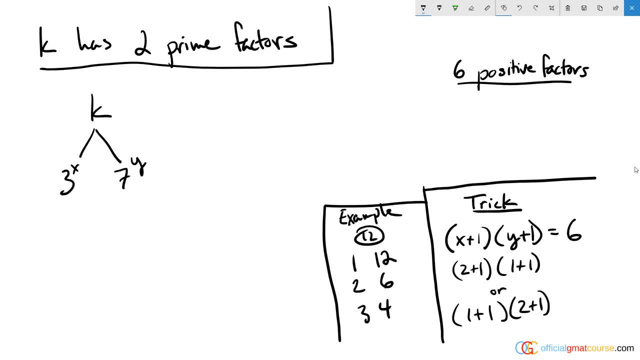 of six factors, kind of like the situation we have in this question stem. And another way we could have quickly figured out how many factors 12 has, including the number one and the number 12 itself, would have been to take the prime factorization of 12, which is two squared times three to the one. 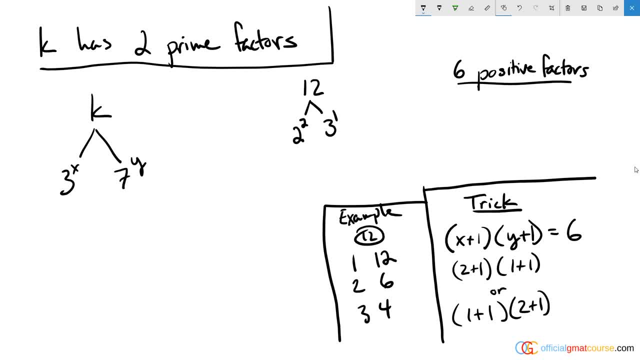 so it's four times three. take that prime factorization and then take each of the exponents from the prime factorization and if you have more than two factors, two prime factors, you would take as many prime factors exponents as you have, but we're going to just 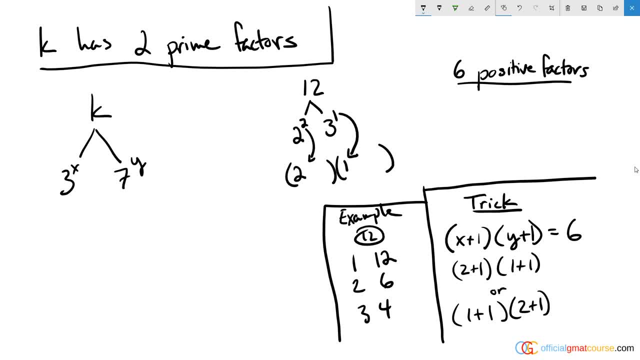 take these two, because this is all we've got. you take those prime factors, you add one to each of them and you multiply them together, and what we get here is three times two, which equals six. and this is just a trick. this is just something to put on a note card and memorize. it's a quick way to 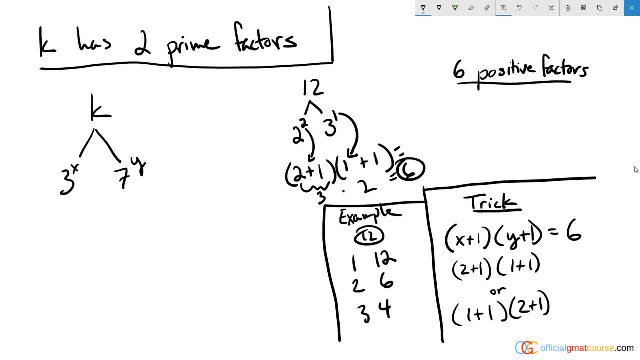 find the number of factors that a number has based on its prime factorization. so if we know that k has six uh total positive factors, including one and the number itself, and we know that k can be represented as three to the k times seven to the three to the x, times seven to the y, because we're told that k 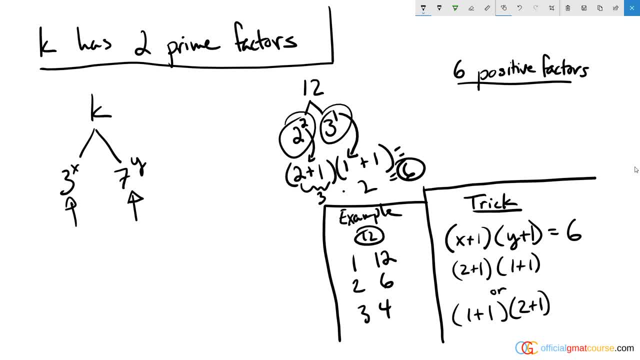 has factors of three and seven, um, and we also know that x and y cannot equal zero, because they wouldn't tell us. yeah, we have a factor of seven, when it's seven to the zero, which just equals one. so we assume that x and y both have to be. 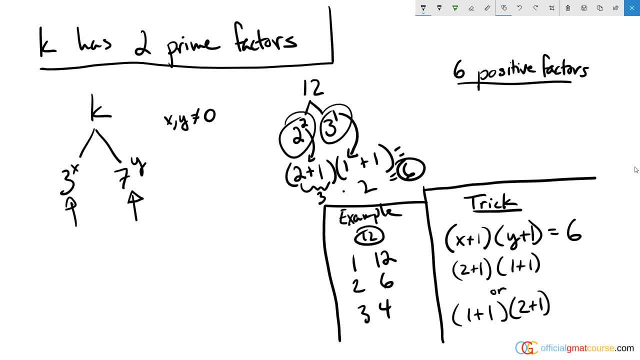 positive numbers. neither of them. they're not fooling us- and making one of them zero, then that means either x is equal to two and y is equal to one, or x is equal to one and y is equal to two, because if we look at the trick that i outlined down here, if we know the total number, 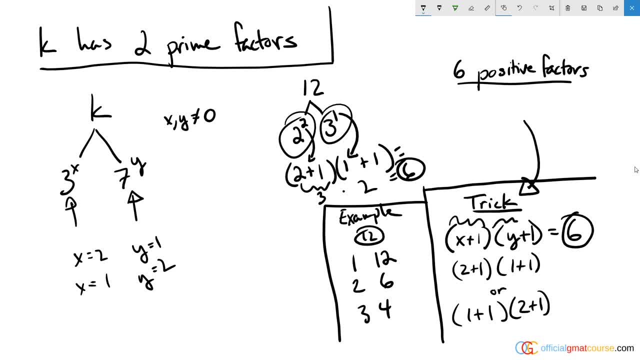 of factors is six, and x plus one times y plus one, which are the exponents on our prime factors, give us the total number of unique factors. then x plus one times y plus one has to equal six, and these have to be whole numbers because we're dealing with a positive. 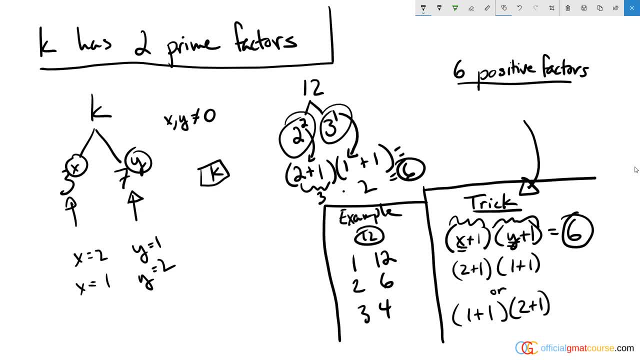 integer for k, and that means that we have a positive whole number up here, which would only make sense if these two things multiplied to give a whole number. so, for example, having both of them as whole numbers would be a way to guarantee that, especially if we have exactly six factors. so 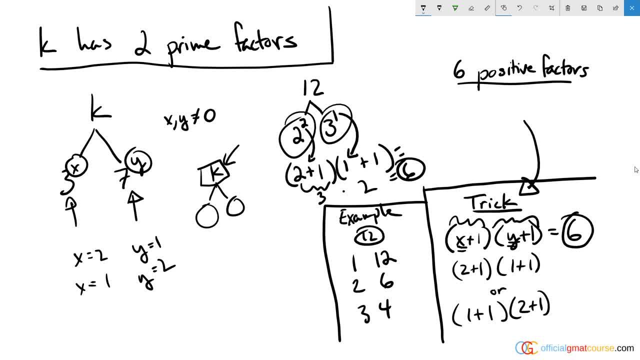 we know that the prime factors are three and seven, then we know that either x is two and y is one, or x is one and y is two. looking at statement one, it says three to the two is a factor of k. well, that means that the x has to be two and that means the y has to be one. and if i know that, the 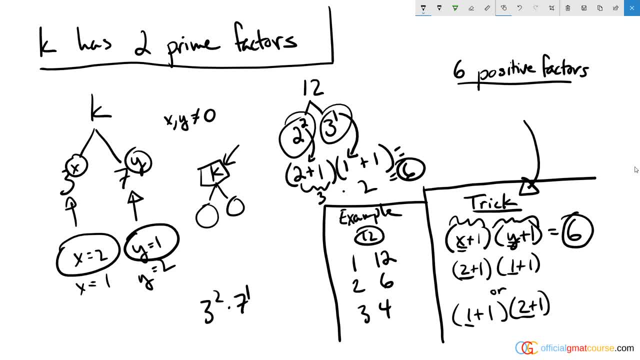 factors are three to the two, times seven to the one, then i know that this is nine times seven, which is equal to sixty three the second. so statement one is definitely sufficient. statement one sufficient. statement two says that seven squared is not a factor of k. but we know seven is a factor of k and so 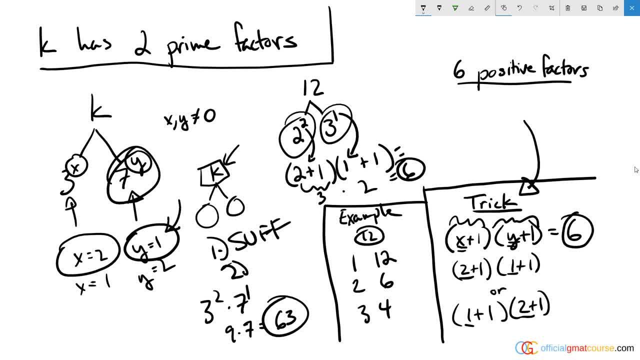 that must mean that the y is equal to one, because the only alternative option given this situation was for y to equal two. but we know seven squared is not a factor of this number, so it must be seven to the one. so that tells us that statement two also gives us the same information as statement one. 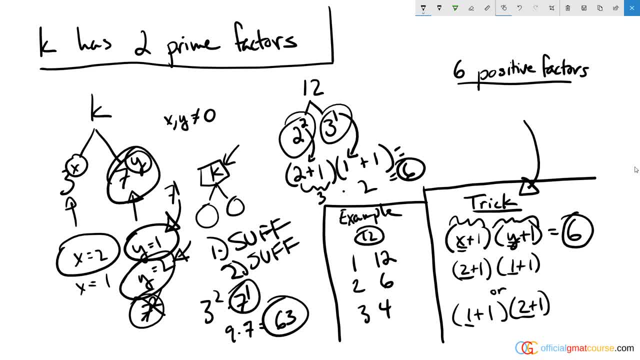 and it's also sufficient. we know that it's seven to the one and then we must have three to the two paired with it, given the info they gave us in the question stem. so there's a little bit of a trick to this, which i don't typically like to focus on tricks, but this is a good, useful one to put on a. 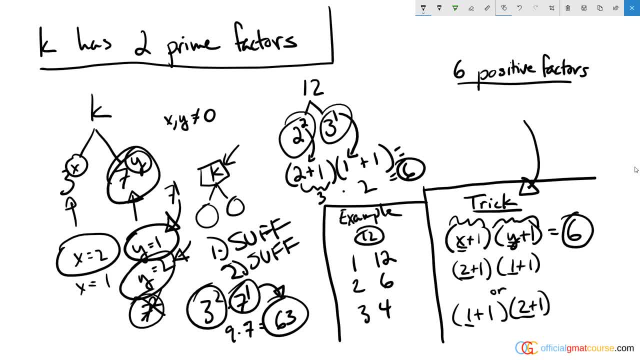 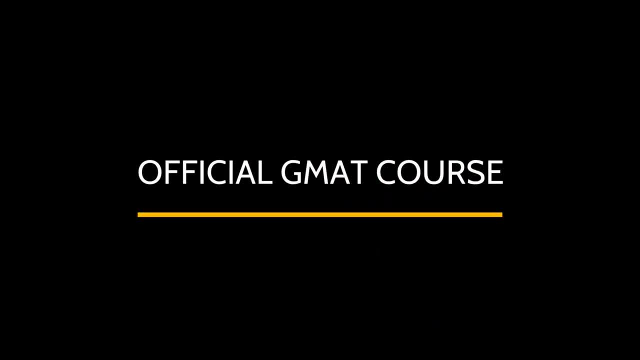 note card. um, i think that it's probably difficult to solve this if you didn't know that in advance. so we'll see if we can find a way to solve this problem.